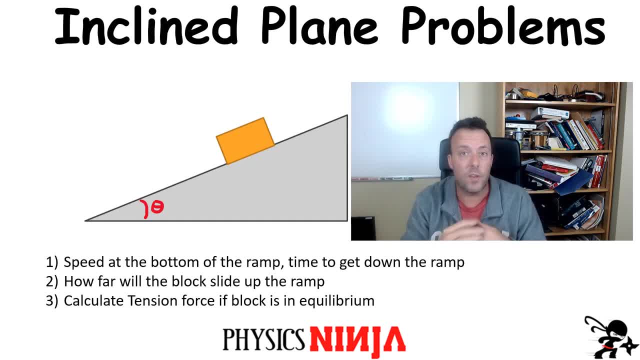 right. So how would I solve that problem? What if there was friction involved in that problem? The last one will be an equilibrium problem. I'm simply going to tie a string to that block, something like this right, And I'm going to connect that to the wall. How would? 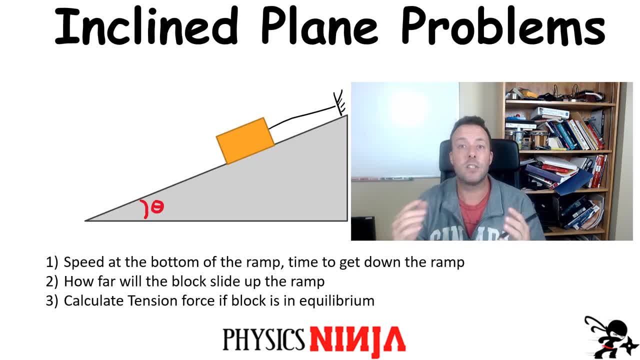 I find, for example, the tension in that string if the block doesn't move, All right. so let's go and get started with these problems. First, let's set up the forces, the free body diagram of the block on this incline plane. I'll show you how to do that in detail, and it's going to set up the 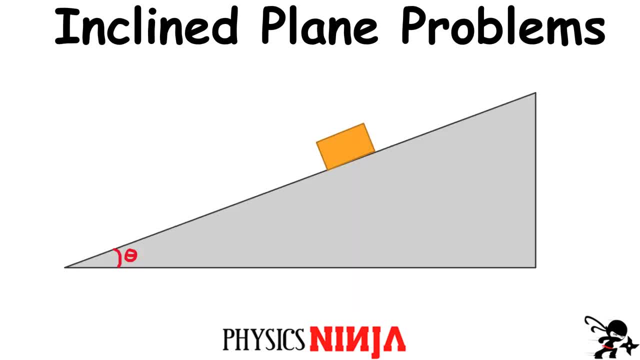 solutions for us. All right, let's get started. All right, we first have to look at a very important force which is always present, And that is the weight of the block. All right, so our block here is going to be assumed to have. 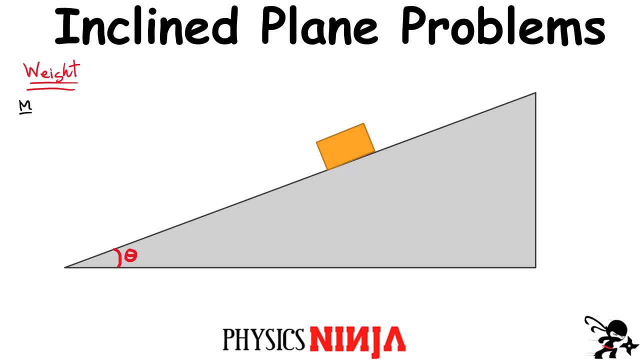 a certain mass. all right, So the mass is simply going to be m. okay, Now the weight. you should know that the weight, you go to the center of mass. you just represent the object by a single point. and now all you do for the weight is you simply make a vector that goes straight down. 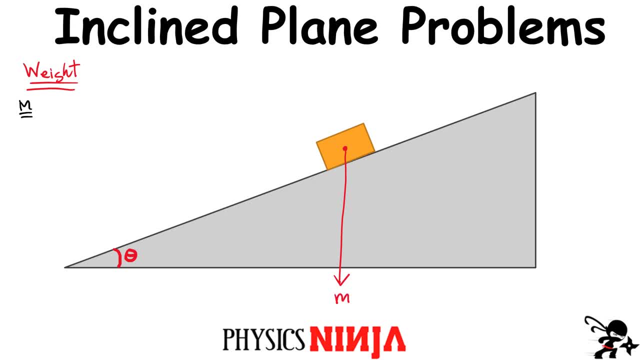 okay, Now the magnitude of that vector is simply the mass of that block. Let's use the same letter, capital, M multiplied by little g. okay, So that is an important force that acts on the block. Now another force that acts on the block is the normal force. All right, so what do we do about the normal? 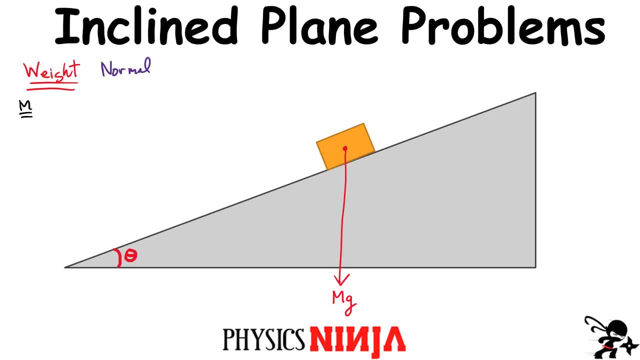 force. Now, in mathematics, normal force, or the word normal, simply means perpendicular to the surface. So let me just write that down: Perpendicular to the surface. in this case, this is the surface, right, The block is resting. So perpendicular to the surface is simply like this, and I'm going to call: 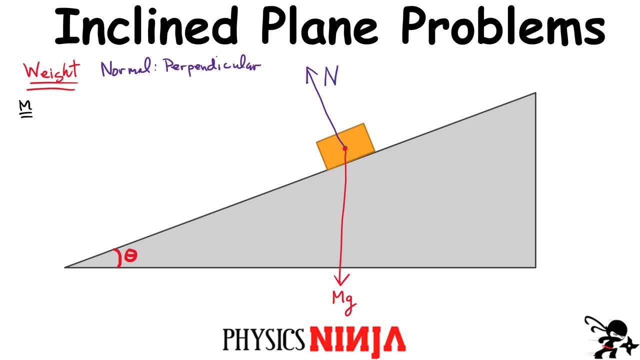 this n for the normal force. Now we see right away, we have a problem, right, We have forces that are not in the same direction, and this one is kind of at an angle relative to the normal. So what do you do in this case? right, It's a little bit harder Now. this is my tip for all of these. 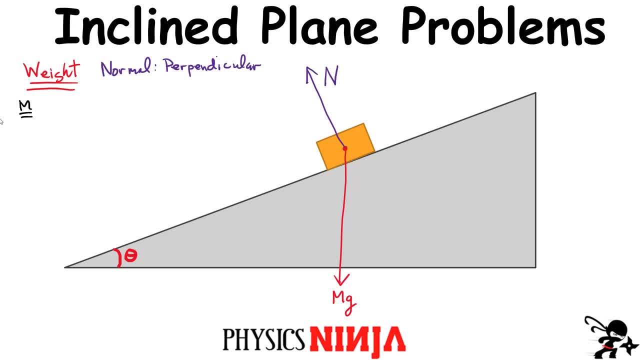 problems. Now, in all problems, you typically have to choose a coordinate system, and mostly we use a coordinate system. So we're going to use a coordinate system and we're going to use a coordinate systems that do this, basically because math has kind of brainwashed us into. 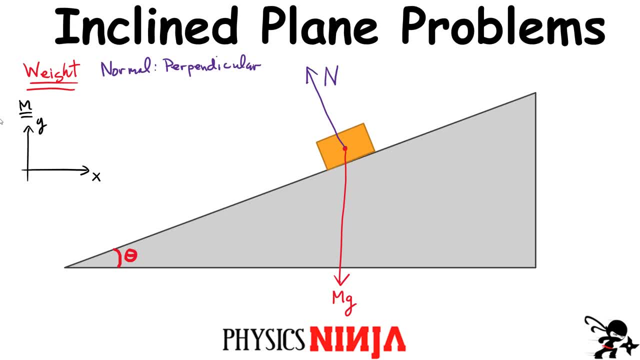 thinking that this is okay And this is okay for most problems. It's actually still okay for this problem. It just becomes way too complicated. So I really don't recommend using this coordinate system. And why not? Well, first of all, if I release this block from rest and there is no, 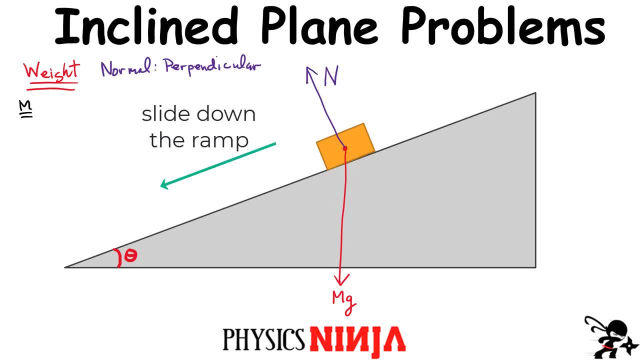 friction, for example, this block is simply going to slide down the ramp. okay, Whenever you have a situation like that, it's always best to use at least one action to get the block to rest. So let's say that I have a axis that is pointing along the direction of the motion. If you know what? 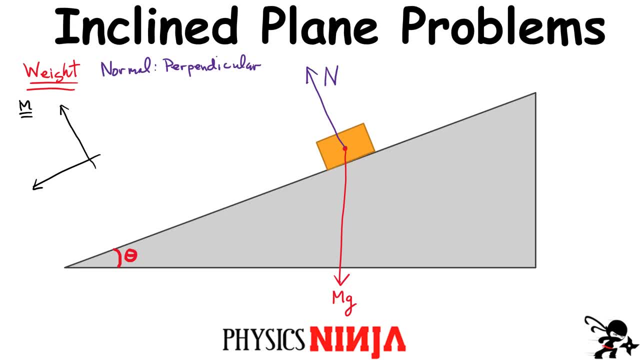 it is. sometimes you don't. But in this case let's just say that the block will slide down the ramp. So I'm going to call the direction down the ramp my positive x direction, and I'm going to call my direction perpendicular to the ramp. I'm going to call that the positive y direction. So right away, 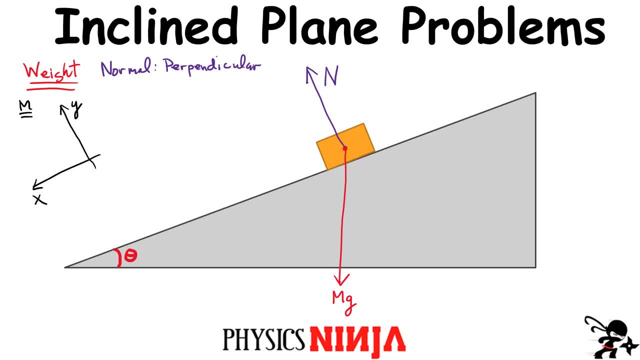 we see that the normal force is simply along the y direction. Now the weight, on the other hand, is not along the x nor the y, But it has a component of each. So our goal now is really to break the weight down into two. 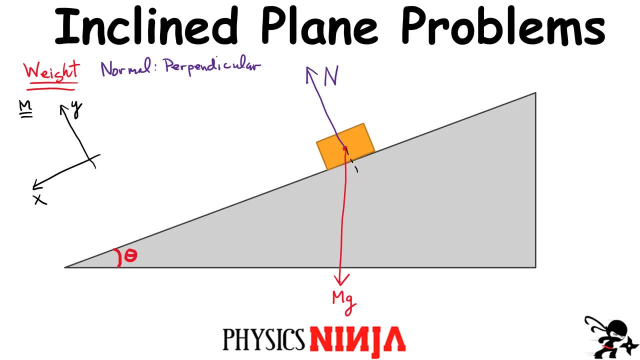 components. And in order to do that, what I'm going to do here is I'm just going to kind of draw in a little bit of the coordinate system. This is kind of like the negative y axis, And I'm going to go ahead and just plot what the x direction looks like for this problem. It makes breaking. 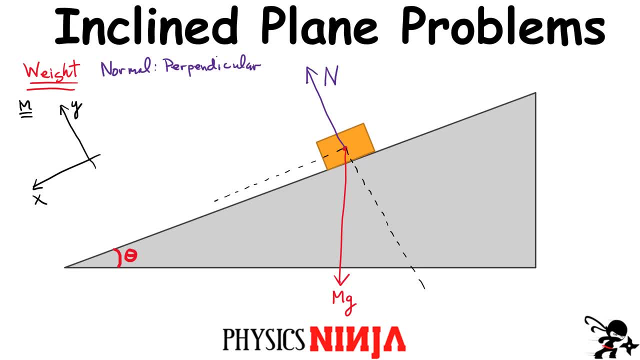 this vector down a little bit easier if you have a clear figure. I find students sometimes make their figures so small it's very, very hard to see the figure, So I'm going to go ahead and see. All right. so if I want to break this vector down into two components, this is what it looks. 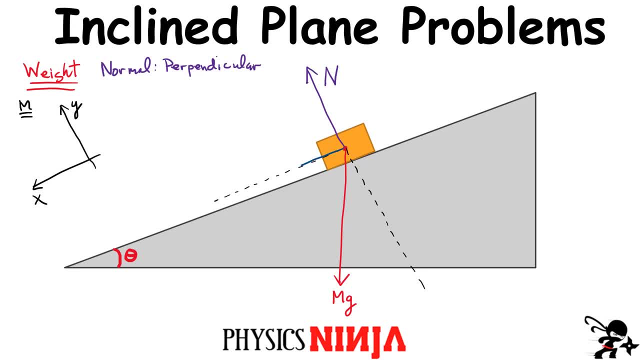 like There should be at least one component of the vector here that acts down the ramp. All right, and if I continue, this here would be again using my coordinate system. this would be the weight that is along the x direction, or the weight that's parallel to the ramp. Now the other. 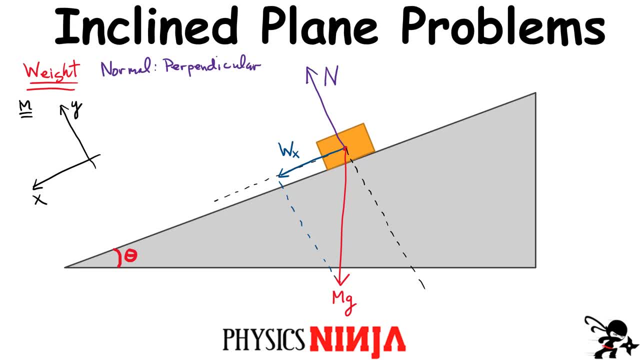 component. let me pick a different color over here. The other component is the weight, a component of the weight that is along this axis, right here, right. This here would be the weight along the y direction, or the direction that is perpendicular to the ramp. All right, let me go. 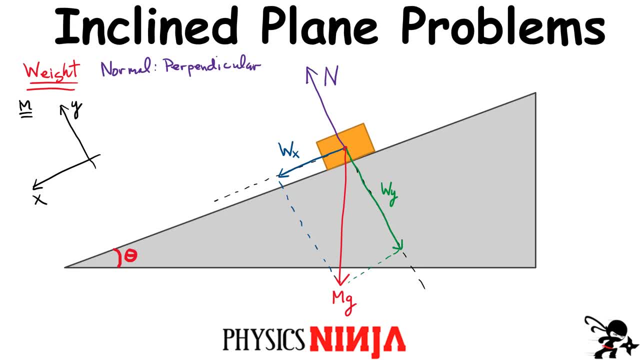 ahead and close off that rectangle here showing the two components clearly. So what we have to do now is, typically, this angle is known. It could be 30 degrees, 20 degrees, I don't care what it is, but typically you know the angle that the inclined plane makes relative. 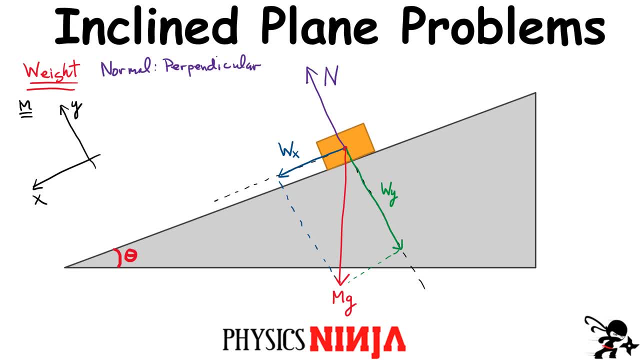 to the flat surface down here. Okay, what we need to do now is figure out, out of all of these triangles, where is this angle, theta? Okay, so what we're going to do here is: let me grab a different color and we're going to highlight some of the different triangles that we could see. First of 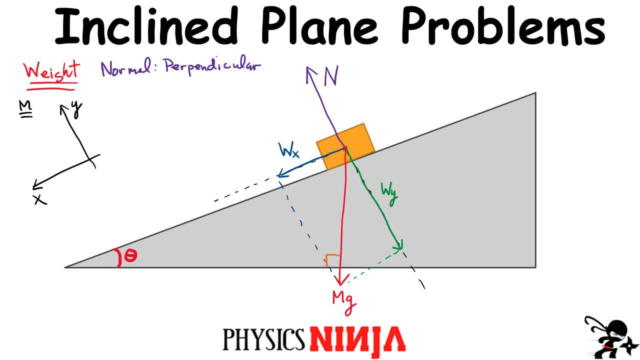 all, if the weight goes all the way down, you should realize that this here should be a right angle, a 90 degree angle, right here, And if you follow this triangle right here, right, the one that includes the angle theta and this 90 degrees, 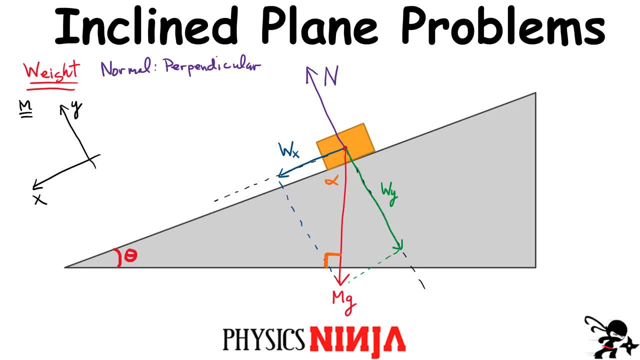 that means whatever angle this is up here, I'm going to call it alpha. is I really have to have that? alpha plus theta must be equal to 90 degrees Because at the end of the day, I end up adding a right angle to that. 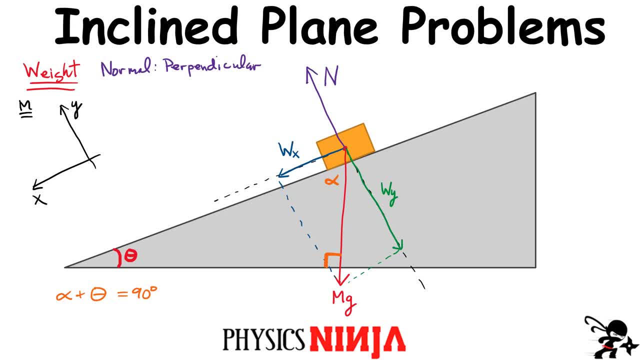 and I know, if I sum the three angles of a triangle, those should be 180 degrees. So that means that the two other angles should be 90 when I add them. All right, so we've done a lot of work. So, for example, if we know that this angle, theta- 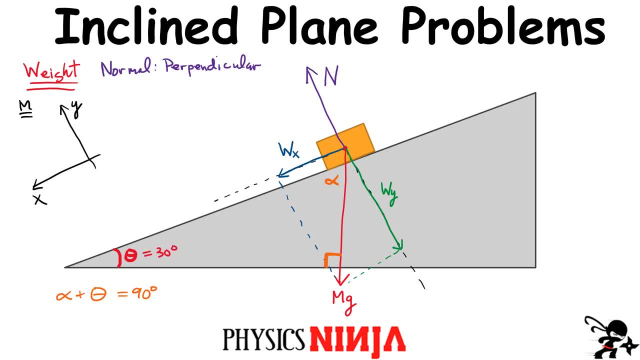 here is 30 degrees, I automatically know that alpha has to be 60 degrees, right in this particular case, Because both of those 30 plus whatever has to be 90. So it must be 60.. All right, I'm going. 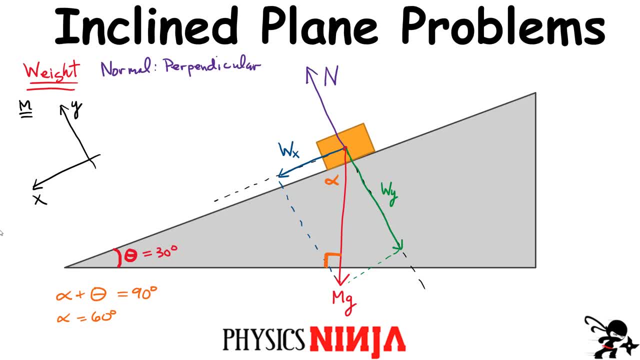 to go one step further now. Now again, if I look at two angles now between the weight in the x direction and the weight in the y direction again, this is also another 90 degree angle over here. So that means, if this here: 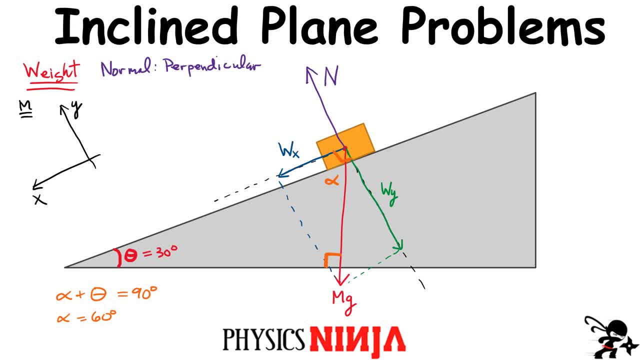 is alpha. you should be able to convince yourself that this angle over here- and this is really the one I like this here's also the angle theta. So if this is 30 degrees, that means that this angle- the way I've drawn it in the figure- should also be 30 degrees. Now, what this allows me to do is 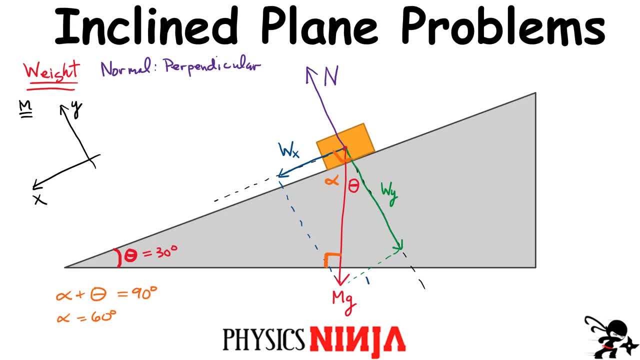 easily write down the components. Let me go ahead and fill out the rest of this rectangle right here. This is the weight in the x direction. Again, the weight is simply the red vector, the hypotenuse of this triangle right here. So let's go ahead and write that. So what would it? 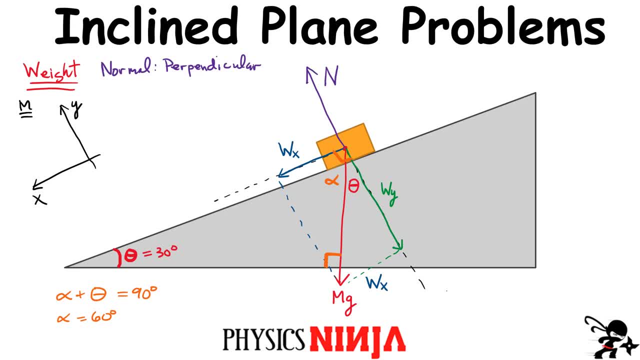 look like for my expressions. So I could write that sine of the angle theta is simply equal to the opposite over the hypotenuse. So that would be the weight along the x direction, the way I've defined it, over the hypotenuse, which is the total weight of the block. So if I rearrange this, 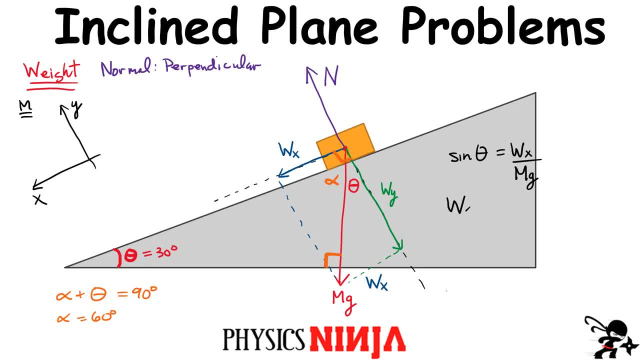 I can get an expression for this component of the weight, the weight which I've called, along the x direction, as mg multiplied by sine of the angle theta. Okay, a really, really important equation right here. Let's go ahead and highlight that one. So that is the component of the weight that is. 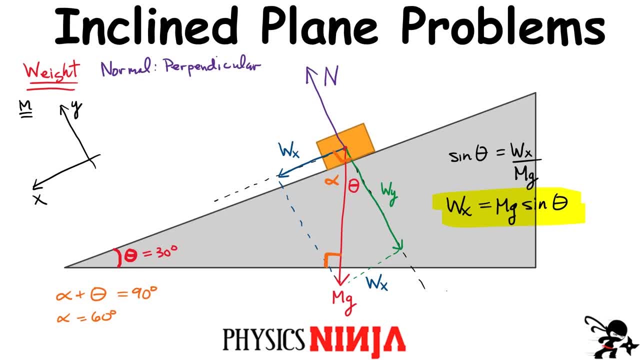 acting down the ramp. Let's look at the other expression. Okay, again, I'm going to use this angle and I'm going to use my triangle. right here I could write an expression for cosine of the angle theta. Cosine of the angle, theta is the adjacent, which, in this case, I'm going to write. 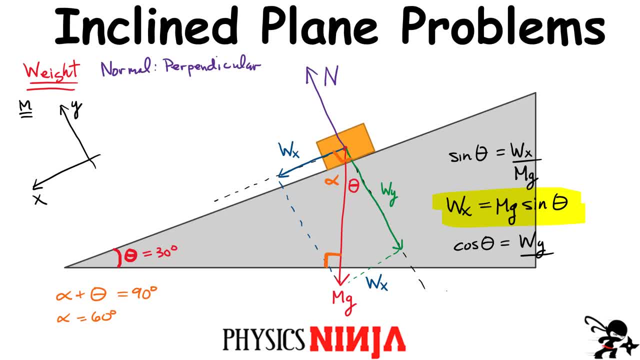 the weight along the y direction divided by the hypotenuse, which again is mg. All right, if I rearrange this equation, I'm going to have that the weight along the y axis is going to be equal to mg multiplied by cos of the angle theta. And this is the second really, really important equation. 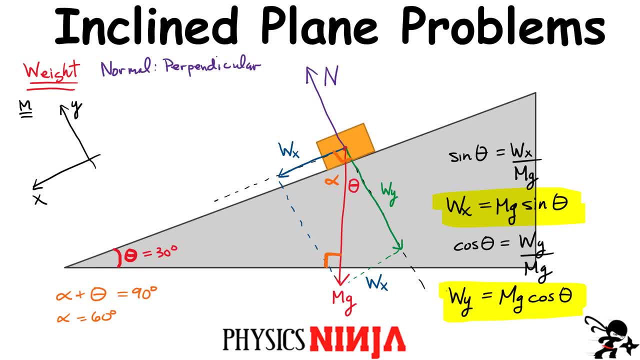 when you're dealing with a block on a slope. If you can understand both of these equations, you're off to a really, really good start right. So we know that this component is the component that is acting down the ramp. So if I rearrange this equation, I'm going to have that the weight. 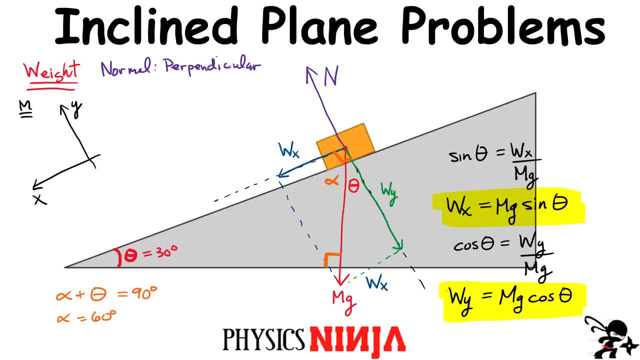 that accelerates the block down the ramp right, Because it's a force acting down the ramp in this case. All right, now let's go back to our three problems. We're going to look at free body diagrams in different cases, but in all our cases we're going to have to break the weight down into: 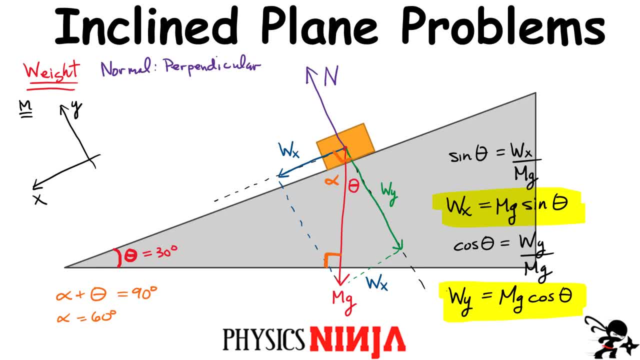 an x component and into a y component, And to analyze most of these problems, it's usually always best to use this type of coordinate system right here that I've depicted, where we have one axis that is directed along the ramp and one axis that is directed down the ramp. So we're going to. 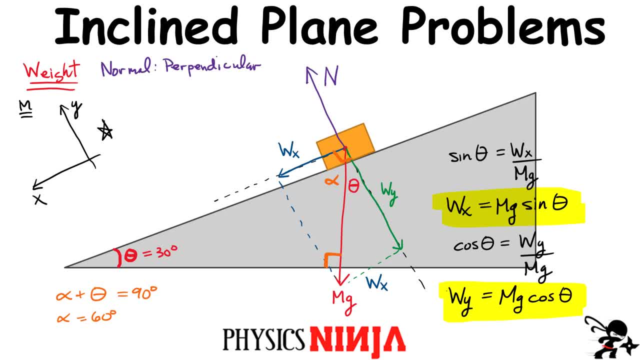 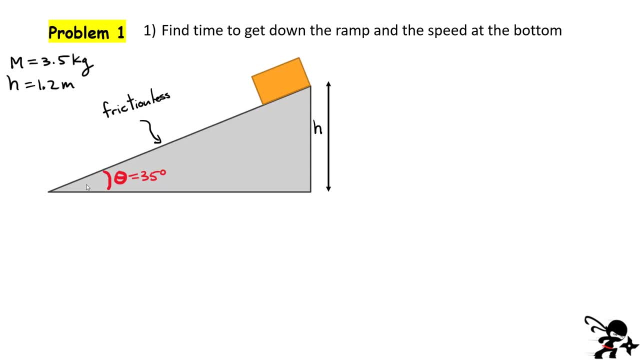 look at free body diagrams in different cases. All right, here's problem one: Let's find the time to get down the ramp and the speed at the bottom. So here's what I have. I have a ramp that has a height of 1.2 meters. My block has a mass of 3.5 kilograms. It's a frictionless surface. 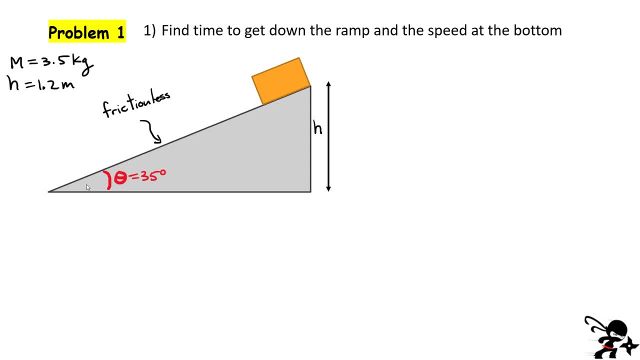 and the angle that the ramp makes with respect to the horizontal is 35 degrees. All right, so let's set this problem up. First thing you have to do is a free body diagram, All right. so, again, just like we did before, we have our weight, which is acting straight down. 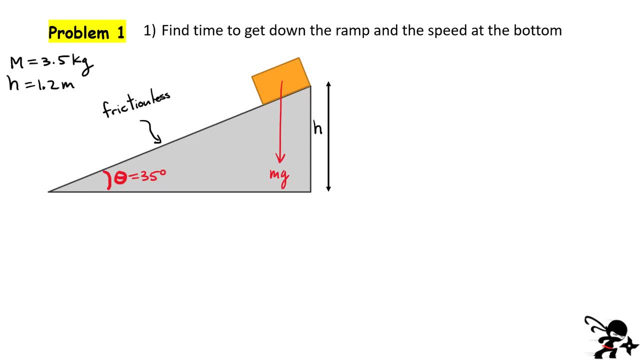 That has a magnitude mg, And we shall also have a normal force in this problem. That is, the surface of the ramp pushing up on the block perpendicular to the surface. That is something we call a normal force. Now my physics ninja tip was to consider a coordinate system where the block is moving like 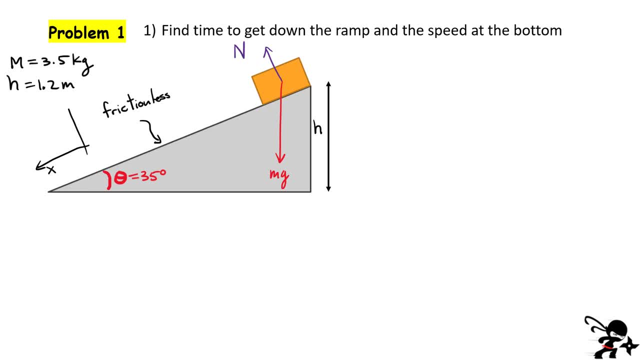 this. So we're going to choose the x direction to be down the ramp and I'm going to choose y to be perpendicular to the surface of the ramp. Now again, if we remember what we previously did, we wrote that the weight can be broken down into two components. I call this the weight in the x. 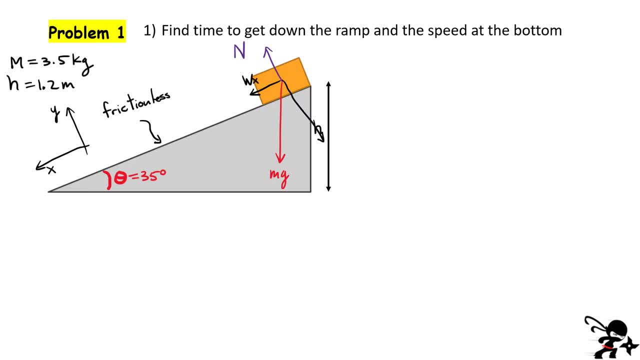 direction and this here was the weight in the y direction. All right, and these components, if you remember what we just did, this was mg sine of the angle theta, sine of 35 in this case, and this guy here was mg cos of the angle theta. 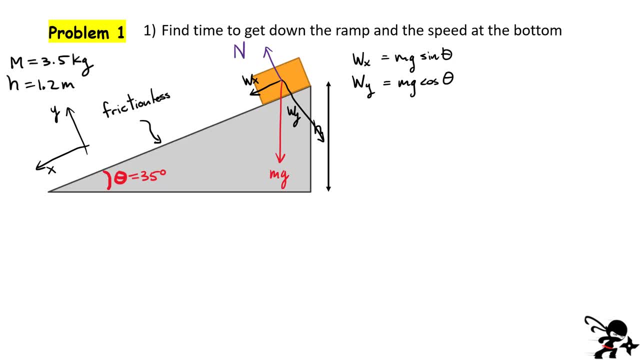 All right, the next thing I really have to do, let me clean up this kind of vector right here. The next thing I want to do is I want to write down Newton's laws of motion for this block. okay. So what that means is I want to write down the sum of the forces along both axes. 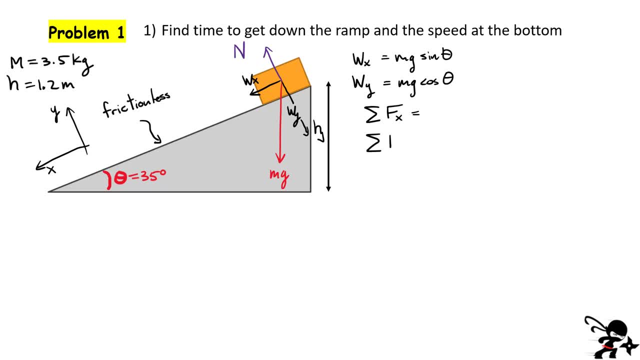 okay, Sum of the forces along the x direction and the sum of the forces along the vertical direction. Now, along the vertical direction, we have two forces: We've got the normal force and we've got this perpendicular component of the weight. 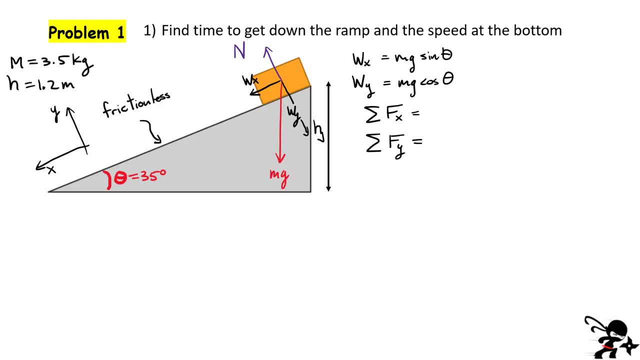 Right, Those forces. when I add them up, they probably have to sum to zero, right? Otherwise the block would fly off the ramp or into the ramp, and that's not what is going on. All right, and how about in the x direction? In the x direction, we only have a single force, right? 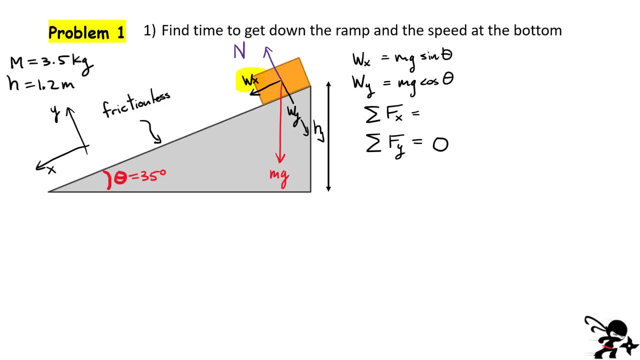 We only have wx, so it's not going to be equal to zero. It's going to be equal to the mass of the block multiplied by the acceleration right. This is Newton's second law at work, right here, All right. so what does this term look like? Well, 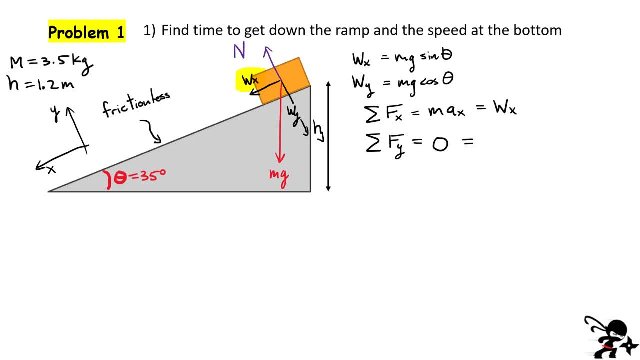 this is simply equal to wx In the vertical direction. we've got two, so we've got the normal acting up- I'm going to call that positive n- and we've got the weight in the vertical direction acting down. right, That's this component of the weight acting down. Okay, now I'm going to 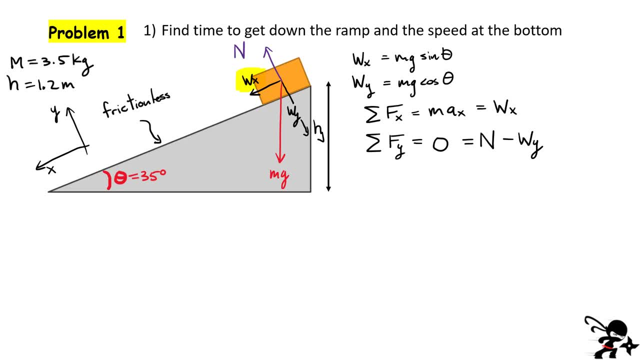 substitute my values of wx and wy. So let's go ahead down here. So we have mass times. acceleration in the x direction. This here equals mg, sine of the angle theta. Now look what I have. I have mass on both sides. Well, guess what? I could eliminate that one. 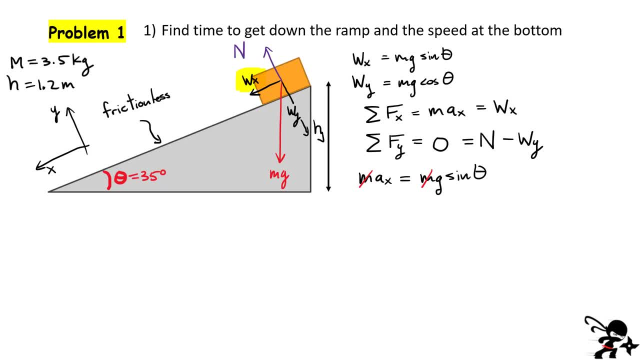 and now I'm left with just one expression for the acceleration in that direction, parallel to the surface of the ramp right. The acceleration ends up being g sine theta. Let me highlight that That's an important result. We're going to use that in just a minute. 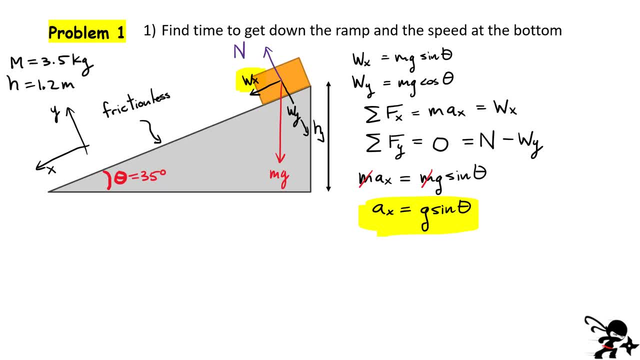 to do some kinematics. Let's have a look at what we get in the vertical direction. So that's using our second equation here for forces In that direction. we're going to have mass on both sides In that direction. we end up finding that the normal force is simply equal to the weight in the 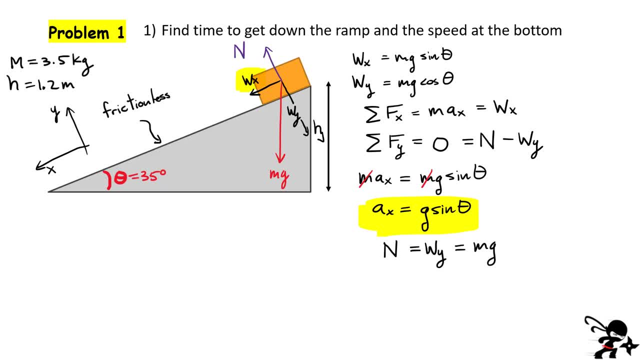 vertical direction. So that is mg cos of the angle theta. Okay, so we now have an expression for the normal force. In this case it doesn't really help us, but later on, if we look at a friction problem, we may need to calculate what the normal force is. All right, let's go ahead now and 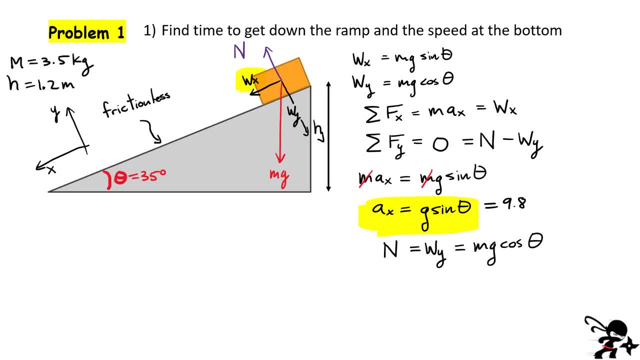 calculate our acceleration. So we get 9.8 for the acceleration due to gravity, little g, and we get 9.8 degrees. I substitute everything in here. I should get around 5.62 meters per second squared. All right, let's go back now to our original question. We're looking for the time. 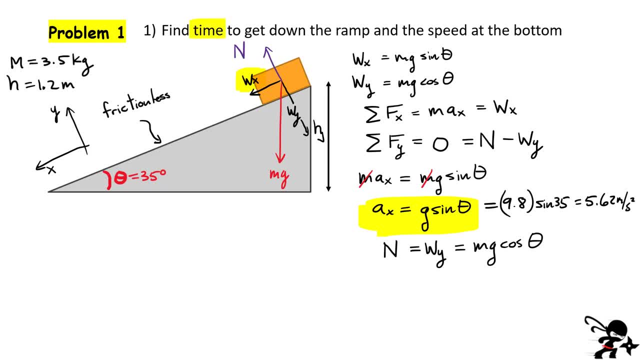 How much time does it take to travel this distance? Now, we're not specifically told that distance. However, we are told the height, So maybe we could calculate that distance right. Let's have a look at the triangle right here. All right, this is really the distance that we're. 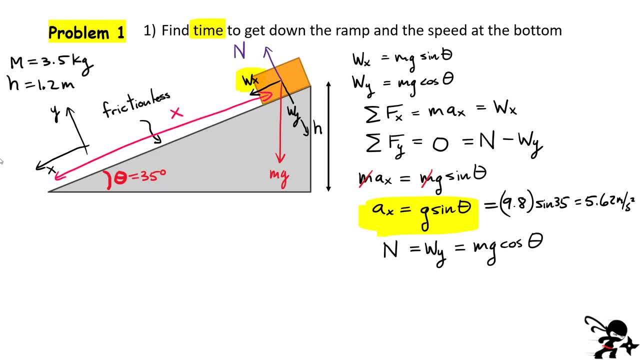 looking for. We're going to call this distance x. I think if we use a little bit of trigonometry we should be able to figure out an expression for that distance x right? Imagine: here you use sine of 35 degrees, because x is simply the hypotenuse of that triangle, h is the opposite side. so this is: 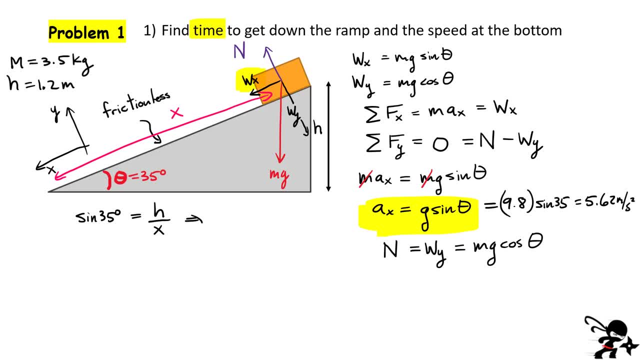 simply h over x, which means at the end that x is going to be h over sine of theta or sine of 35 degrees. All right, so we can actually go ahead and calculate that This is 1.2 meters and this here is. 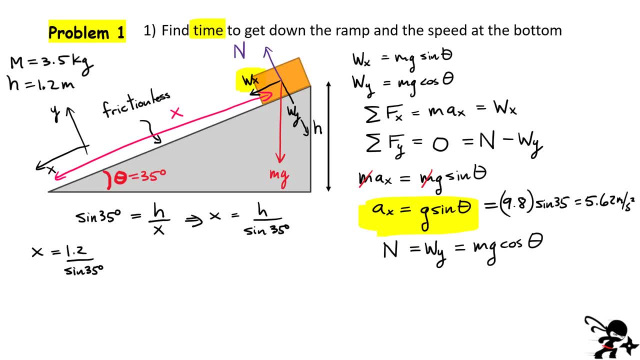 sine of 35 degrees. Anyway, you can actually get an expression for that. I'm not too concerned with that right now. Let's go ahead now and find the time. So how would you find the time? We know an acceleration, We know the distance that we want to travel here. I could just put that in the 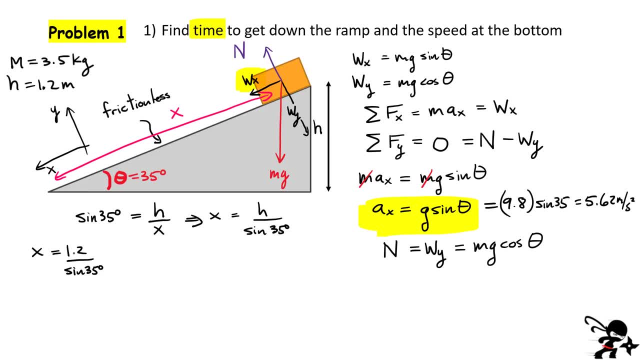 calculator and evaluate it. So now we're going to use our kinematic equations. All right, and one of our kinematic equations, if you remember, should look like this: All right, that my x displacement, all right, delta x, or I'll just call it x in this case, is equal to: 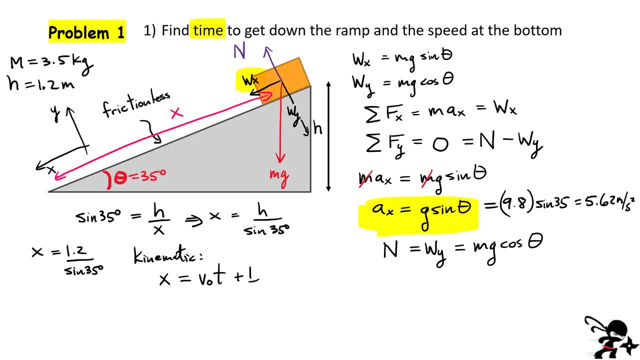 the initial velocity multiplied by time, plus 1 half the acceleration multiplied by t squared. Now, in this case, remember, we're starting from rest, so the initial velocity term is equal to zero, And all I'm looking for here is how do I solve for this time? So we're going to do a little bit of algebra. 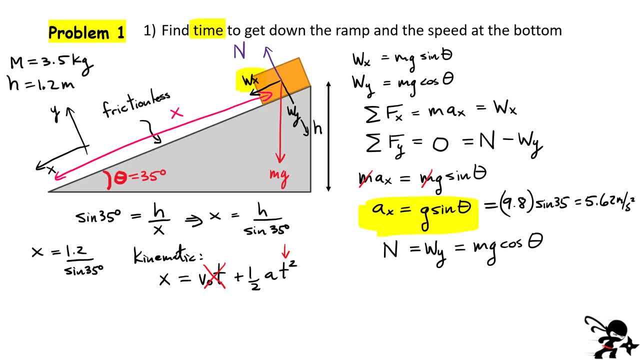 here We're going to get time by itself. So you bring the 2 on the other side, You divide by a and then you take the square root of my expression And I should get something like this: So this is 2x over a, And I can actually take it a step further now and substitute in all: 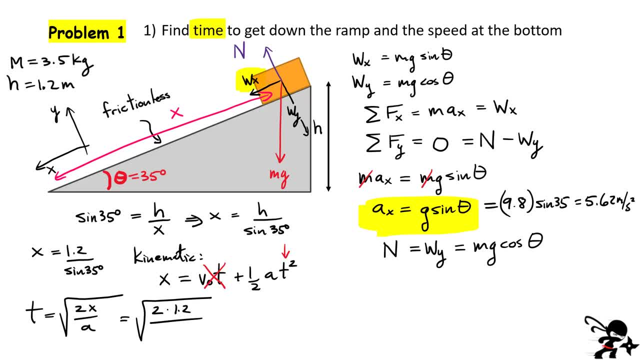 our numbers. My x value was 1.2 divided by sine of 35 degrees, okay, And my acceleration value I calculated earlier- was 5.62.. Putting everything now in the calculator which you should get is approximately 0.86 seconds. All right, so that is the time to go down the ramp. 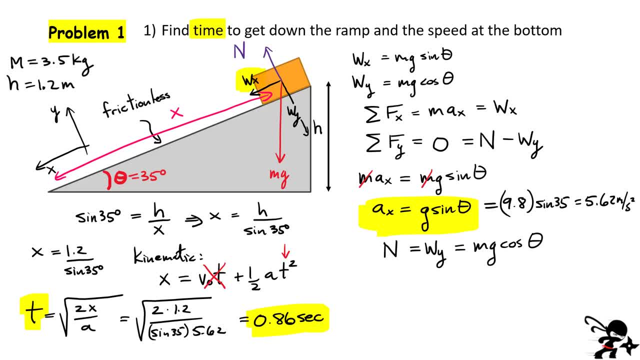 All right, and the next question was: well, what is the speed here at the bottom right? How would I find the speed of the block at the bottom? Again, now that you know the time and you know the acceleration, we have another kinematic equation right, Another kinematic equation. 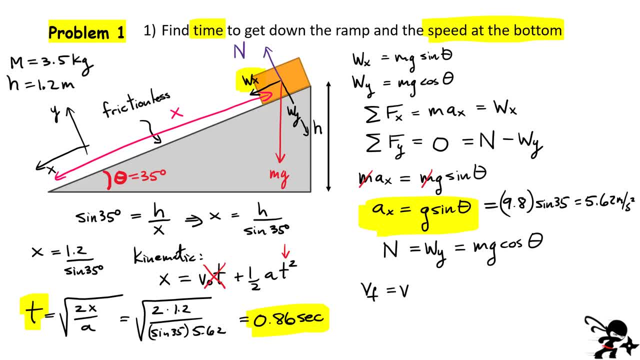 looks like this: that the final velocity is equal to the initial velocity plus acceleration multiplied by time. All right, so again, we're noting the fact that we're starting from rest, so forget about this guy. And now, well, you simply substitute in our numbers, So we get 5.62. 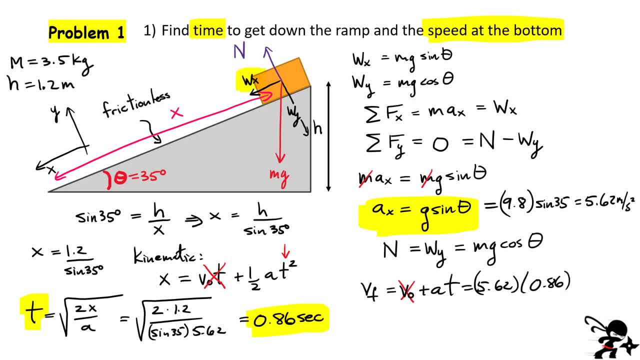 multiplied by 0.86 for that particular problem, And my final speed at the bottom would be 4.83 meters per second. Okay, so kind of a nice starting problem. Let's go look at something a little variation of this problem. 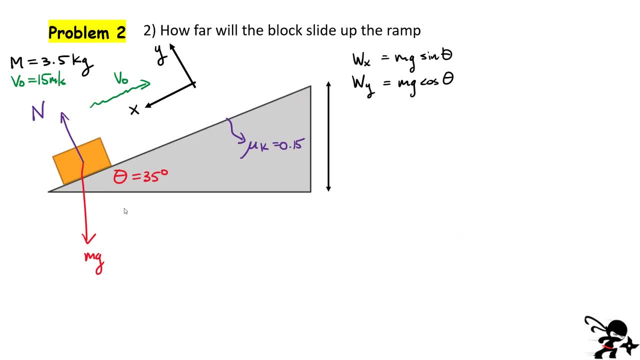 Problem two: All right, problem two: we want to know how far will the block slide up the ramp. So in this case here, I'm giving it an initial velocity of 15 meters per second, And in addition to gravity, what I'm going to do here is I'm also going to put friction on the surface between the 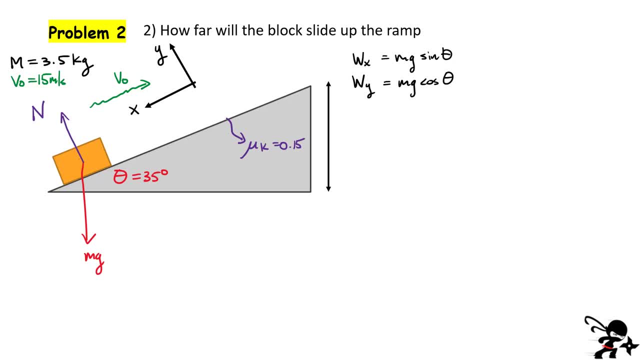 block and the ramp. So that means we must add another force to the free body diagram of the block. In this case, here I'm going to add an additional force. This here is the force of friction, and I'll call it F sub k. So I'm going to add another force to the free body diagram of 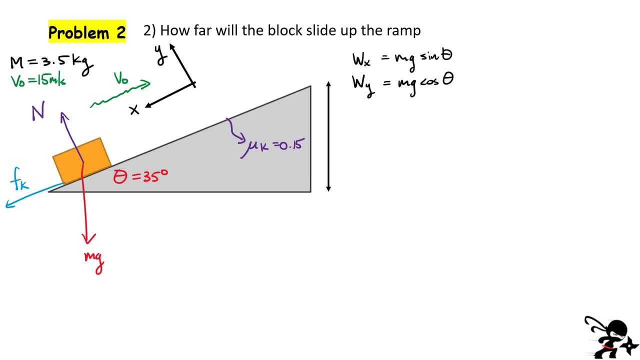 F sub k for kinetic friction. All right, I know the components of the weight so I can go ahead and just add those to my diagram. if I wanted to right, The perpendicular component of the weight, which I call w, y goes like this, And the weight along the x direction should look like this: 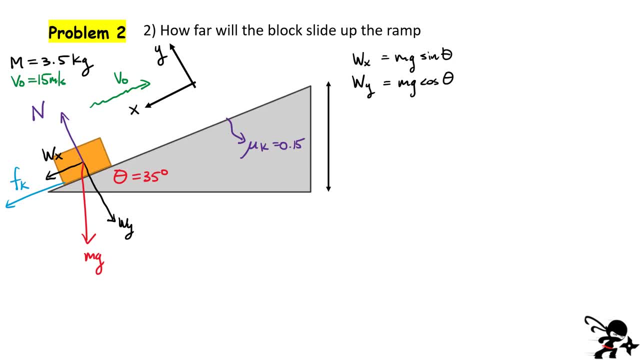 All right, so what are we going to do now? Well, let's go ahead and apply Newton's laws to this problem. Okay, so we're going to have the sum of the forces along x direction. Again, they're going to be equal to the mass times the acceleration of the block. Now look at my two forces along the x. 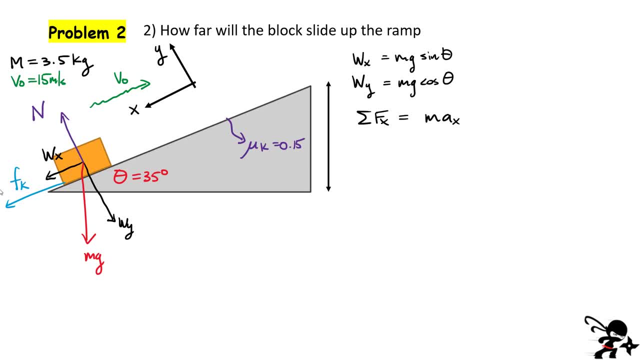 direction. They're acting down the ramp. So guess what? The acceleration is going to be down the ramp. Let's go ahead and evaluate this. So I get the weight along the x direction, plus the force of kinetic friction must be equal to the mass times the acceleration of the block. So I could take 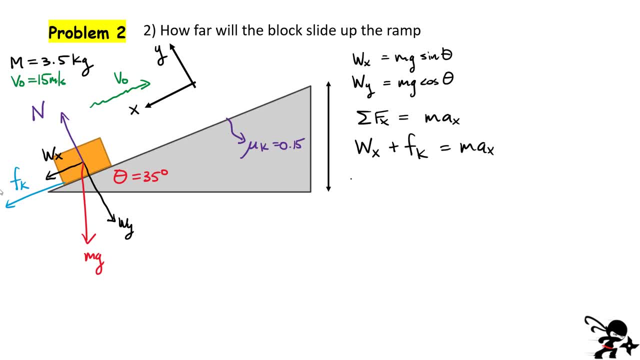 this expression a little bit further now, because I could substitute my value for the weight in the x direction. We have mg sine of theta. And what is the kinetic friction? So kinetic friction, you should remember from your class, this one, is a coefficient of kinetic friction multiplied by the 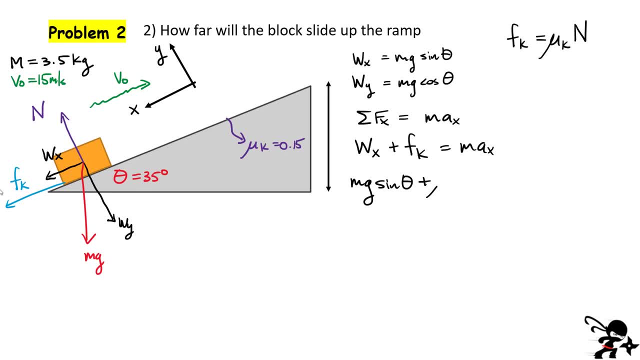 normal force. All right, so let's go ahead and write that. That's our coefficient of kinetic friction. In this case it's 0.15 multiplied by the normal force, And that must equal to the mass times the acceleration in the x direction. So in order for me to calculate acceleration, I need one. 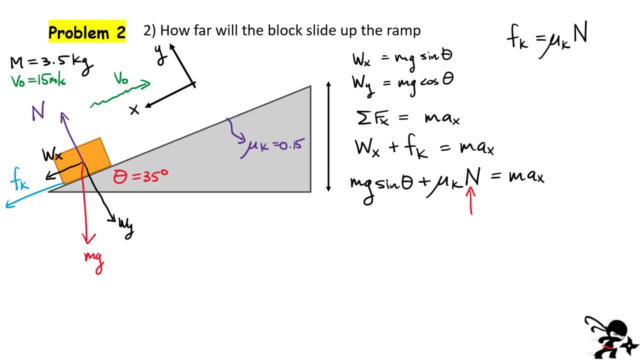 thing Notice: I have the normal force here. So how do I get rid of the normal force to get just an expression for the acceleration in the x direction? Well, to introduce the normal force, I'm going to use the forces in the vertical direction. So let's go ahead and do that right. So if I add up all of 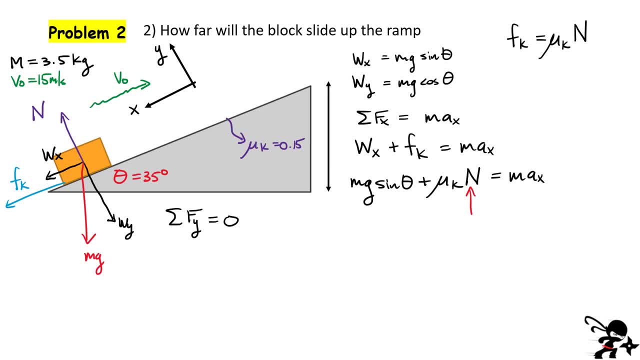 the forces in the vertical direction. I know that those should be equal to 0 because the block is not flying off the surface or going into the surface. So that means you must have that, the normal minus the weight in the y direction. So I'm going to use the forces in the vertical direction. 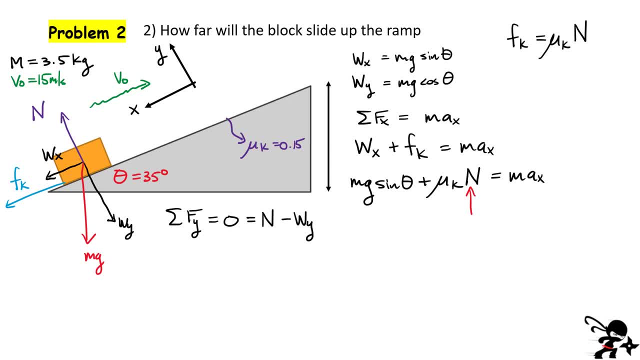 in the y direction should be equal to 0. And at the end you could simply write that the normal force is equal to the weight in the y direction, which we know is mg cos theta for a block on a slope. Okay, so let's go ahead now and simplify this. What we're going to do is substitute this: 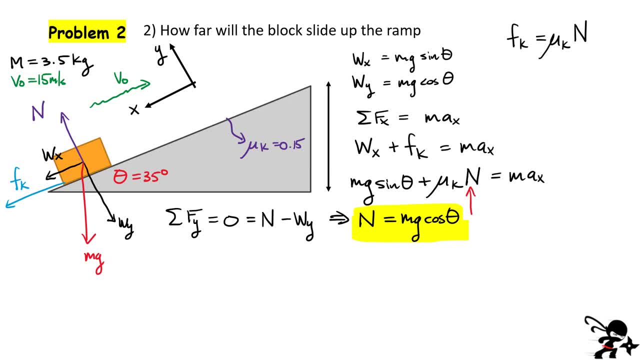 normal force expression into the Newton's second law to find the acceleration. So let's go ahead and do that right down here. So this is kind of a lengthy expression. Let me switch the order here. So I'm going to write the mass times. acceleration equals to mg sine of the angle theta and then minus. 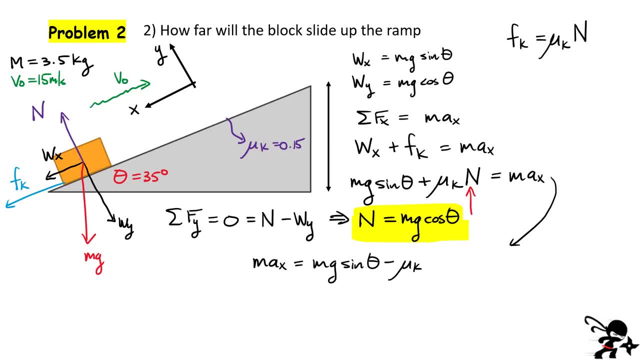 this coefficient of kinetic friction. And right here for the normal force, I'm just going to substitute that with mg cos of the angle theta. That's kind of a lot of algebra there. Next thing we do look at, the mass is included in every term, So I can actually just eliminate it. And one last: 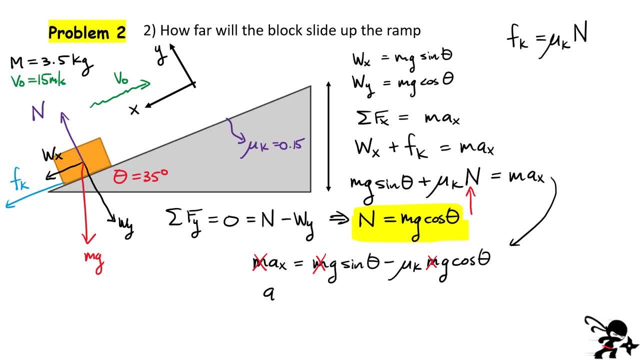 step I'm going to do, just to tidy it up a little bit- is simply to write that the acceleration in the x direction I'll factor out the mass times acceleration. So I'm going to do that, And then I'm going to add a little g, And then this is just kind of a simple expression or simpler looking. 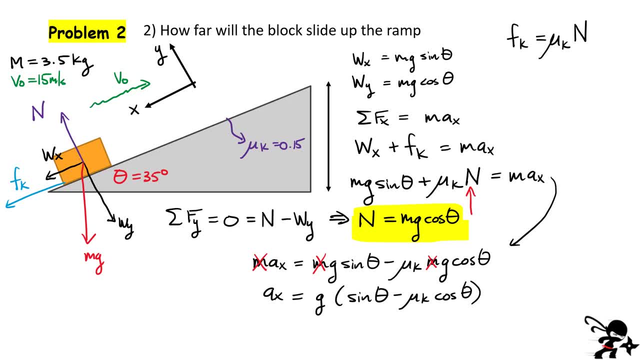 expression than the previous one I had. Now I could substitute in all the numbers to get a number for my acceleration, So this here is 9.8.. What else? We have 35 degrees, So you could substitute that in there. We have the coefficient of kinetic friction, which is a 0.15, and then 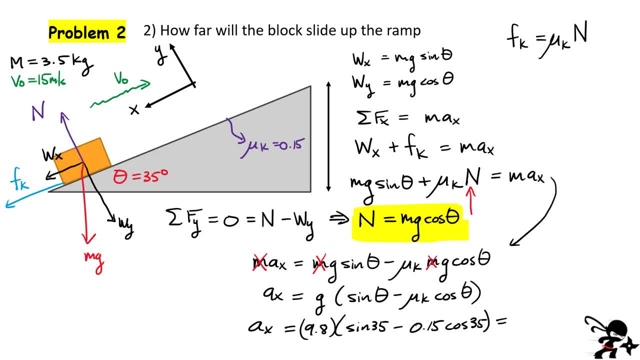 cosine of 35 degrees. Now, assuming I did that correctly, I put that in the calculator- I should get the equal to 0.83 meters per second squared. Notice, I get a positive number right And positive is simply indicated by this direction. The positive x direction is actually down the ramp. 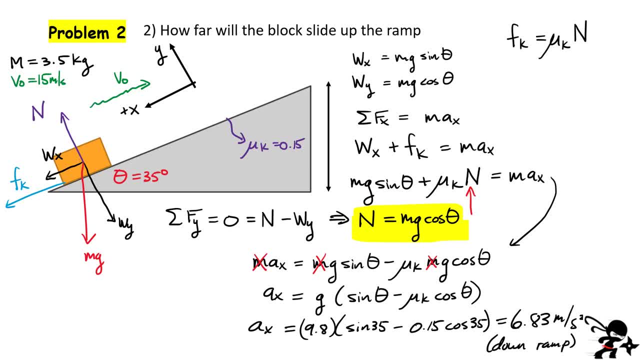 right, So down ramp. That's the direction of my acceleration. Now my initial velocity was going up the ramp, So now I want to know how far am I actually going to go? So I want to know: what is this distance over here that I'm going to travel? right, We can call this the distance over here. 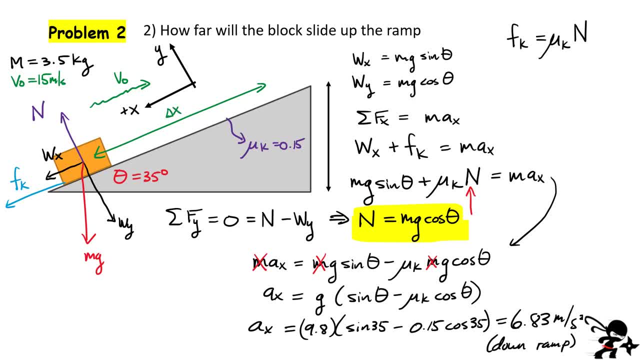 call this, say, the x displacement over here. How far am I gonna go Now? what's special about the maximum height that I'm going to reach is that my final velocity here should be equal to zero at the end of the day. All right, so again, we're gonna use. 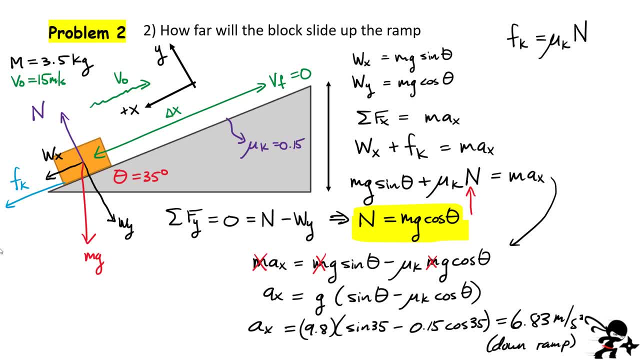 some kinematic equations. okay, If you remember one kinematic equation, I'll just write it as kinematic equation here. One popular kinematic equation was this: v final squared equals to v initial squared plus two times the acceleration multiplied by the displacement. 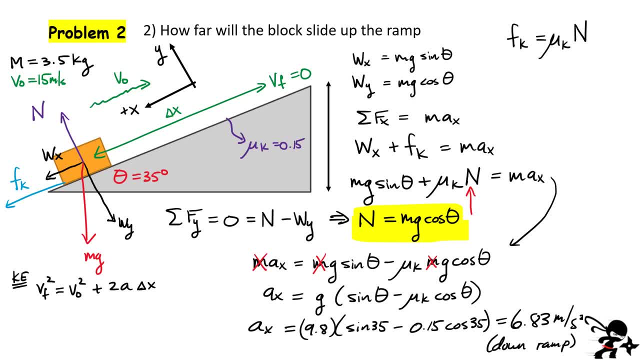 All right. so one thing to remember now is that my displacement is actually a vector that goes from the start all the way to the top, So this displacement here that I'm going to get at the end of the day is going to be a negative number. 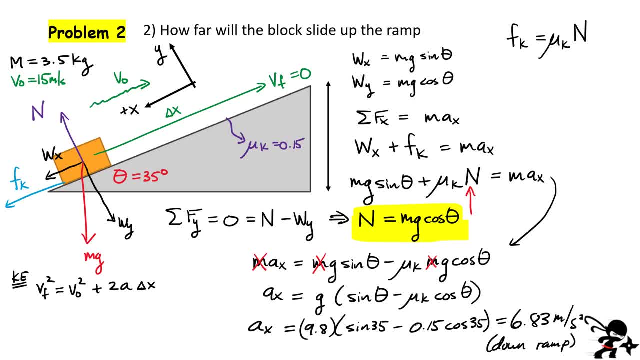 because this is my coordinate system and that's okay. The final velocity. I know that this guy here should be equal to zero. My initial- I've been told it was 15, so I could substitute that in there and I just solve for the acceleration. 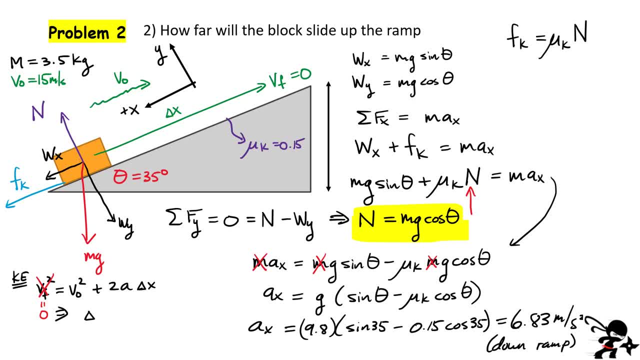 So at the end all we have to do is solve for delta x. So delta x equals to minus v, zero squared over two a. Now we substitute in all the numbers, so you get minus 15 squared over two times 6.83.. 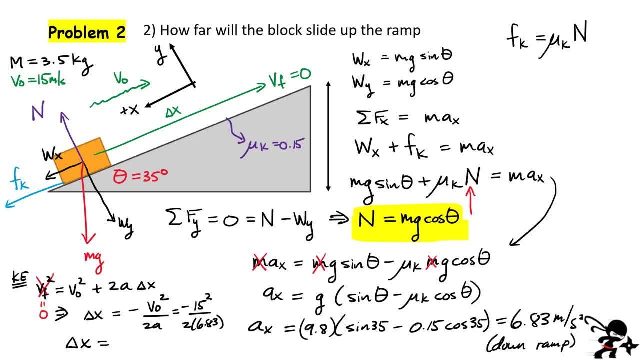 All right, so my final displacement. don't worry about the negative sign, right? the negative sign is only with respect to this coordinate system. okay, So I expect the displacement to be a negative value. All right, if I put everything in the calculator. 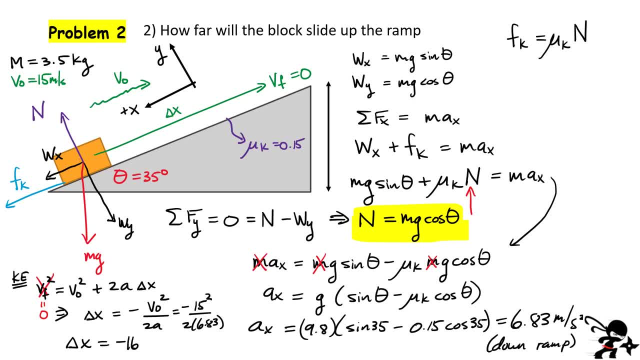 did things correctly, I think I got around negative 16.5 meters as my displacement, And again, this here is only telling me the direction. All right, great. so that's how far you would end up sliding up the ramp. All right, let's look at problem three now. 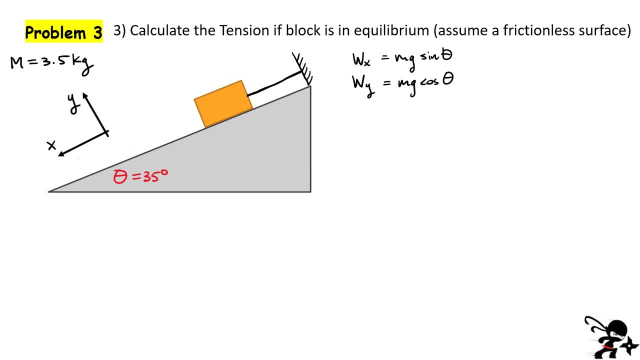 All right, here's problem three: Calculate the tension if the block here is in equilibrium. So what I've done is I've tied a string from the block to a wall- I am assuming a frictionless surface- and that's it. So let's go ahead and start with our free body diagram. 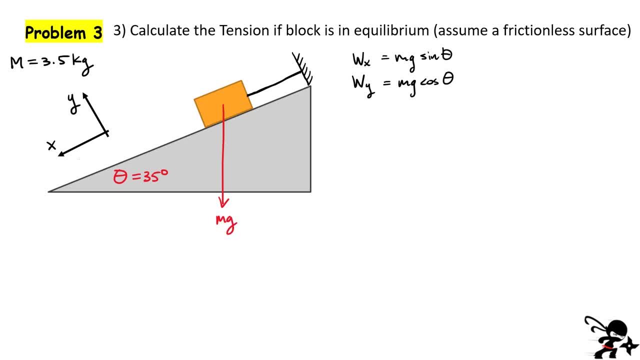 So again we have the weight acting straight down. That has a magnitude, mg. Let's do the easy forces first. We still have our normal force, which is perpendicular to the surface. We now have another force, right, But we have a string attached to it. 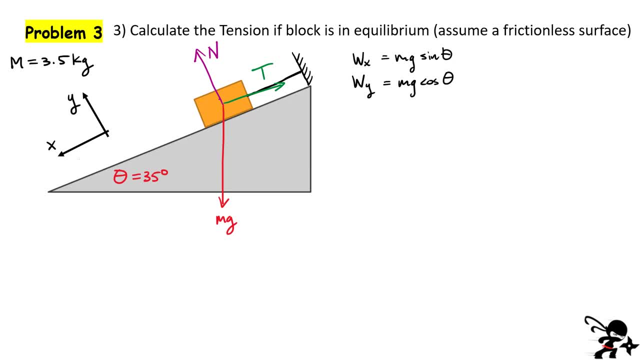 So we have to have a tension force which is acting in the direction of that string. Sorry, my ankle's a little bit off there, And that's it. What we do is we break down our forces using this type of coordinate system again. 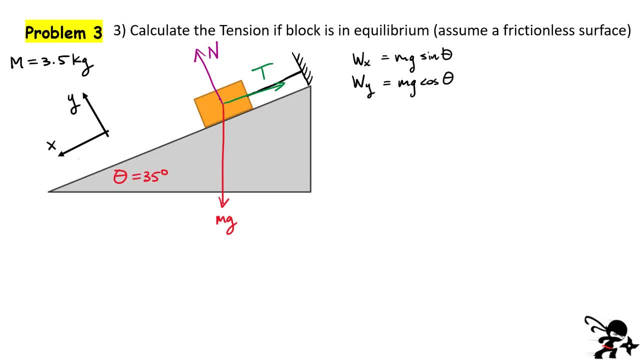 So the normal. we don't have to worry about The tension. if I look at it, it's actually along the negative x direction. All I have left to do here is break the weight down, and this I've done several times already. 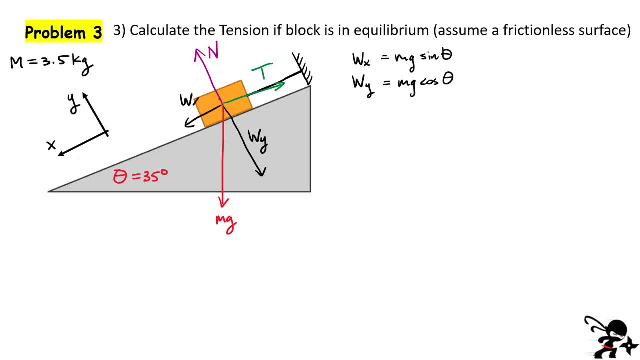 so we should be professionals at this. That's it, That's wx and that's wy. Next thing we wanna do now is simply add up the forces in the x direction Now, in this case here in the x direction, since the block is what